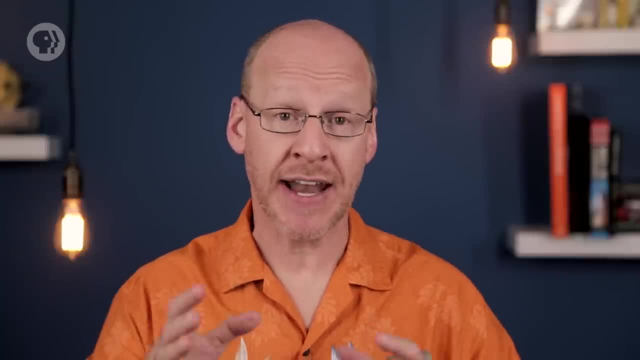 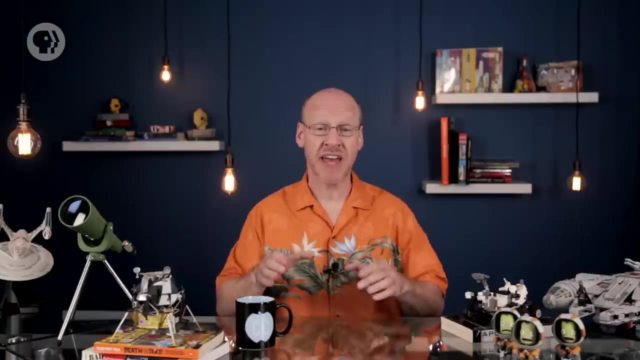 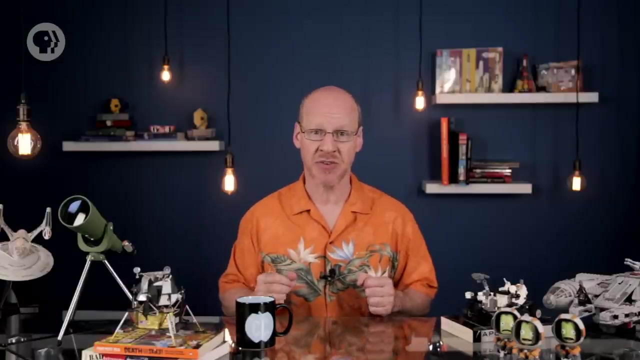 It begins, quite literally, in the grip of Cold War, paranoia, and ends… well, it doesn't end, What true story ever does, But it does lead us to discovering the single most violent events occurring in the universe, events which, paradoxically and ironically, are almost entirely hidden from our view. After World War II, the allies that were the United States of America and the United Soviet Socialist Republic had gone their separate ways. They had fought together against the Soviet Union and the Soviet Union. They fought together against a common enemy. But that war was done and a newer, colder one forged. The US and USSR became sworn enemies themselves, each determined to bring the downfall of the other. Both sides had nuclear weapons, so this downfall was not as impossible as it might seem. It was a terrifying likelihood taken very seriously by everyone involved. Both sides were testing nukes at every available opportunity, pushing them for ever greater. explosive yield. At the same time, both factions were becoming more adept at space exploration, Using satellites to spy on each other, And both were looking at the idea of orbiting platforms from which to launch nuclear weapons. You could lob bombs on the enemy within minutes, instead of needing the better part of an hour. using ballistic missiles. Fear of this, as much as anything else, drove the writing of the Outer Space Test Ban Treaty in 1963, forbidding the testing or use of nuclear weapons in space. Among the signatories were the Soviet Union and the United States. 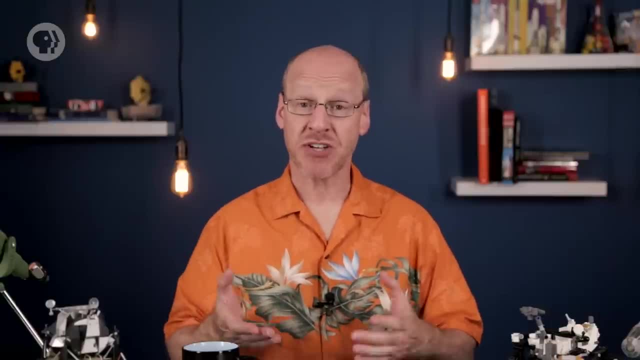 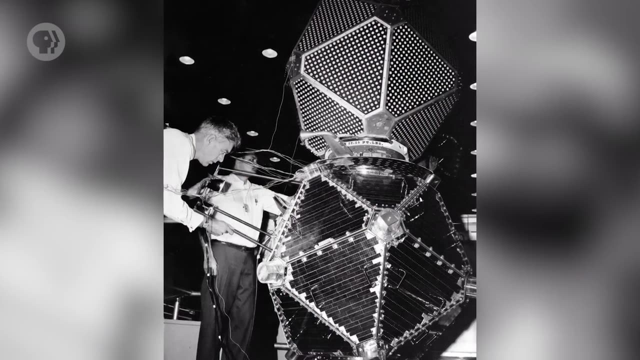 Of course, neither side trusted the other, Fearful the Soviets might try to test any way, perhaps blowing up nukes on the far side of the Moon where they couldn't be detected. the US launched a series of satellites called Vela. Nuclear detonations produce a flash of gamma rays, the highest energy form of light. 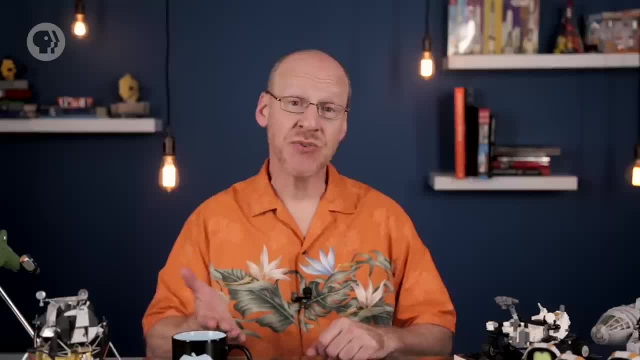 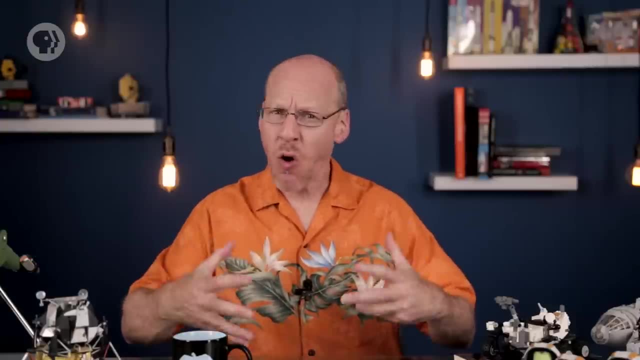 The Vela satellites were designed to detect that high energy pulse. Two scientists, Roy Olson and Ray Klebesaddle, were assigned the task of analyzing the data. They laboriously combed through the observations, checking them for anything that looked like a nuke. Signal after signal turned out to be false. But finally, in 1969, they found their first hit: a flash of gamma rays seen by several of the satellites on July 2, 1967.. But there was one problem: Whatever caused the gamma ray event didn't look like a nuclear blast. 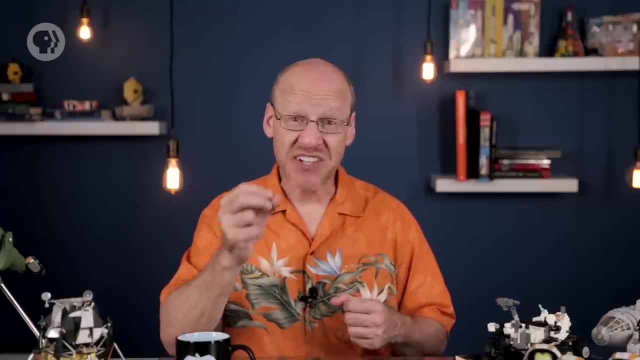 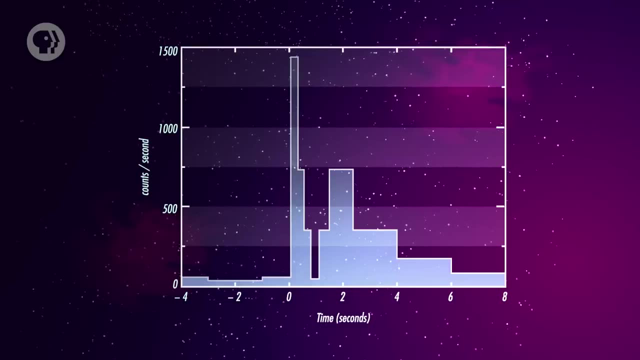 The amount of gamma radiation and how it fades with time are very distinctive for a nuclear weapon, and the July 2 event looked completely different than that. There was a strong, sharp peak of emission lasting less than a second, followed by a longer, weaker pulse lasting for several more seconds. 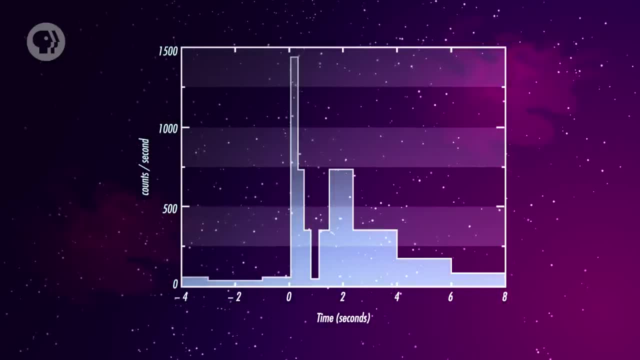 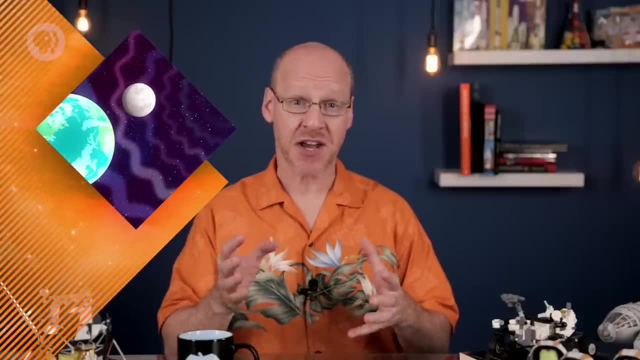 A quick look at solar flare data revealed no activity that day that could generate gamma rays either. Weird. Over time, more and more of these mysterious bursts of gamma rays were found. As analysis techniques got better, it was found that they were not coming from the surface. 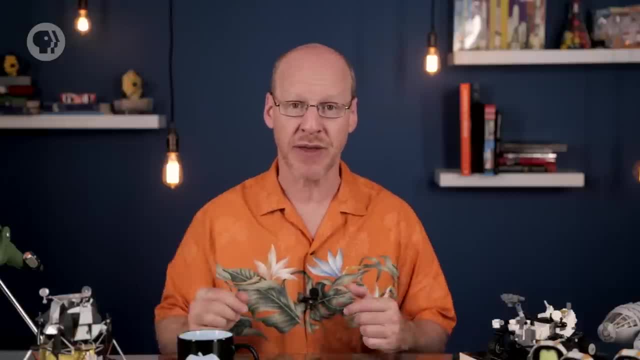 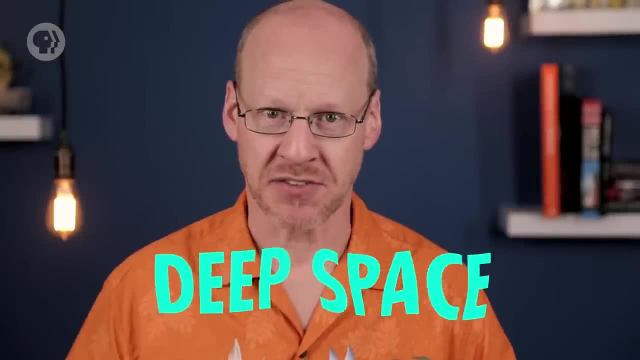 of the Earth, nor from nearby space, that is, Earth orbit. Whatever these bursts were, they were originating randomly in the sky and were happening in deep space. In 1973, Olson and Klebesaddle went public publishing a paper with their results. 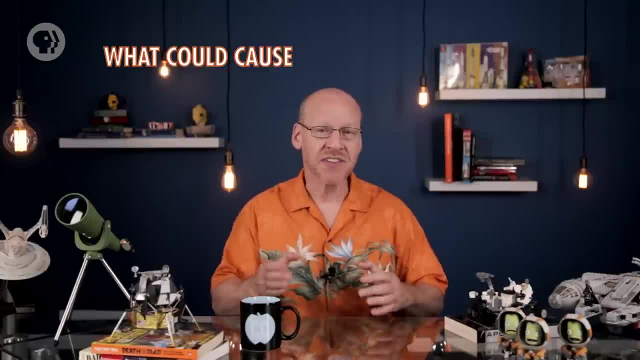 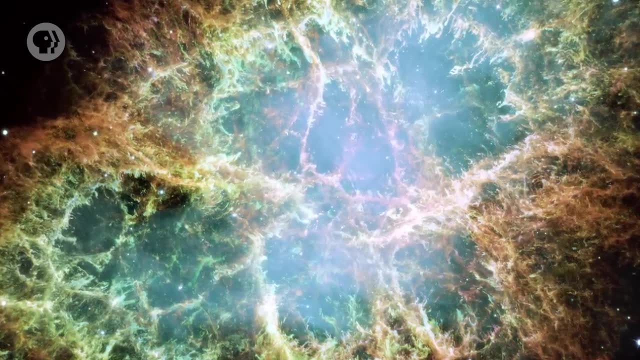 Astronomers were intrigued: What could cause these gamma ray bursts? Generating gamma rays is hard and takes incredibly violent events — exploding stars, massive solar flares and the like. But these bursts weren't obviously associated with any of these events. 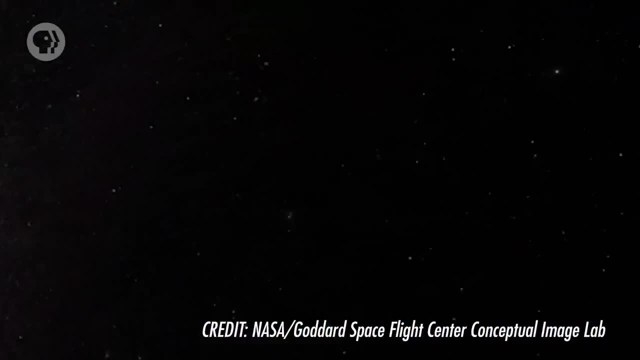 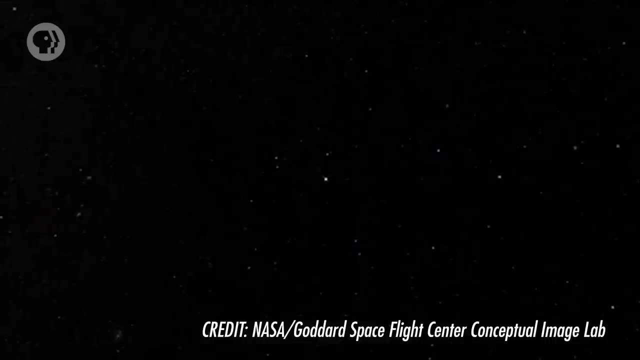 Making it worse. gamma ray bursts — let's call them GRBs for short. okay, GRBs fade rapidly, lasting mere seconds or minutes, making it impossible to follow up with optical telescopes. It took weeks or months after the event to get a position in the sky for them. And even then the uncertainties were huge. At the time, gamma ray telescopes had very fuzzy vision and couldn't pinpoint directions well at all. That meant thousands of stars, galaxies and other objects nearby were candidate progenitors of the detected bursts. 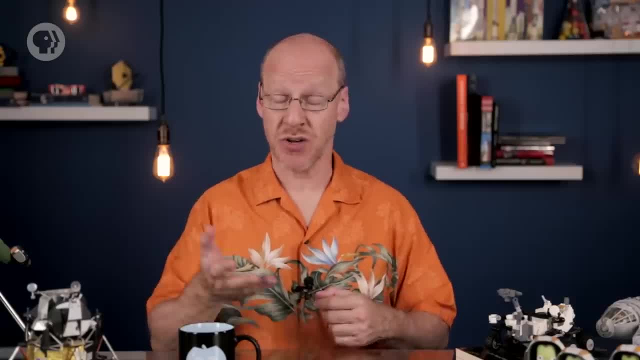 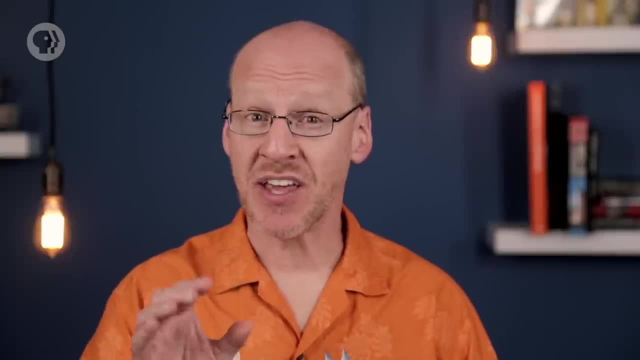 It didn't narrow things down at all. It's like telling someone you dropped a quarter and you want help finding it. When they ask you where you dropped it, you reply Wyoming. As more of these objects were found, it was seen that they really were occurring on random. 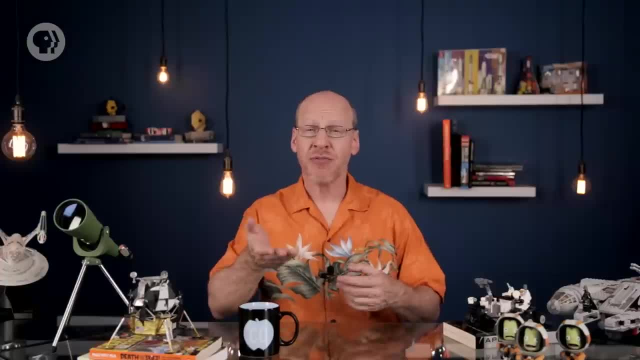 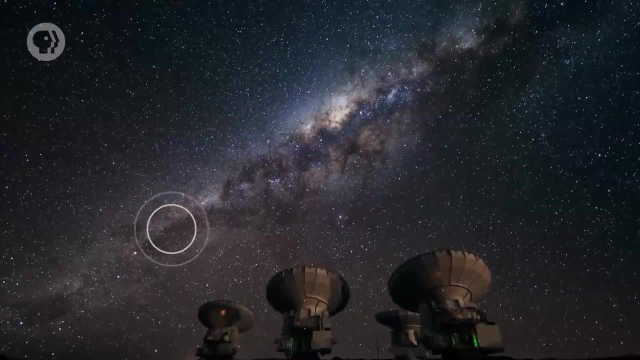 points in the sky, And that itself was a problem. If they were coming from, say, comet impacts on neutron stars, which was one possible hypothesis, then we should see more bursts along the plane of the Milky Way than above it. Pretty much the only place you find neutron stars is in the plane of the galaxy, where 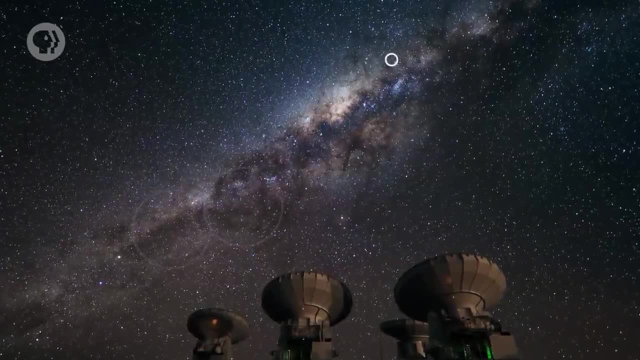 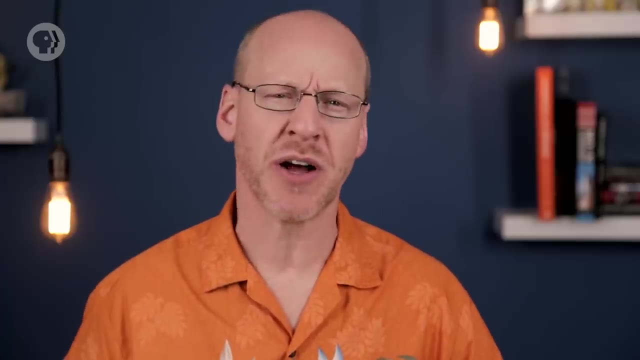 all the massive star formation takes place. If GRBs were from neutron stars, then that's where we'd see them, But we see them all over the sky. That meant GRBs were either very nearby — no more than a few hundred light years — or that they were coming from incredibly far away, So far that even a few hundred light years ago they wouldn't have seen them. Even nearby galaxies weren't affecting the distribution. We didn't see a surplus toward the nearby Virgo galaxy cluster, for example. 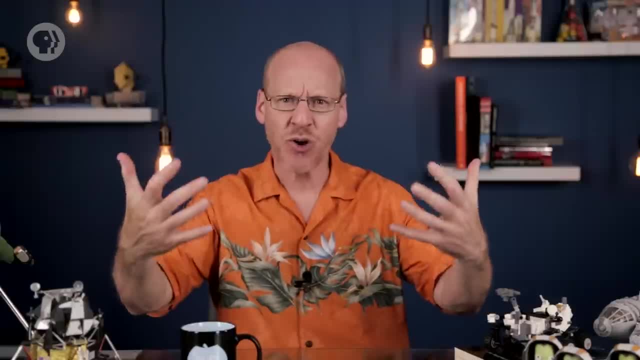 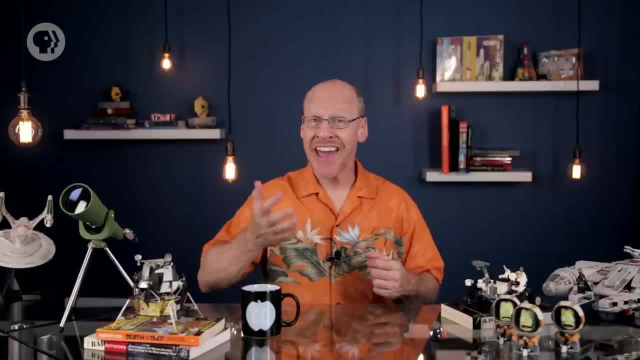 So they'd have to be coming from even more distant galaxies, clear across the universe. Neither explanation made sense, since astronomers couldn't think of anything that could generate bursts that were close by And, obviously, the energies involved in creating a burst of gamma rays from billions of light. 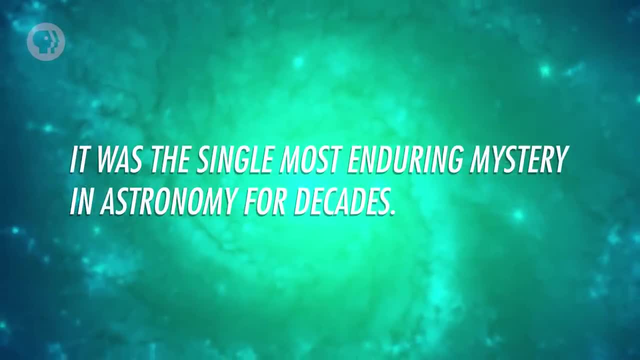 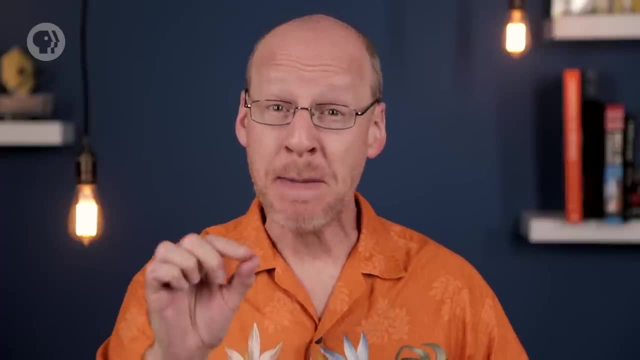 years away were impossibly huge. It was the single most enduring mystery in astronomy for decades. The only hope was to have a faster response time, So that any fading afterglow from an event might be caught before it became invisible. In 1997, that hope became reality. 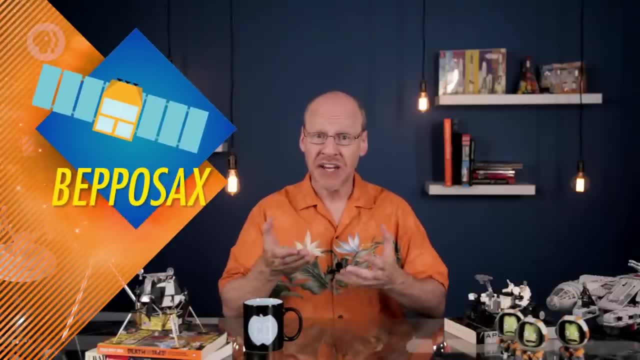 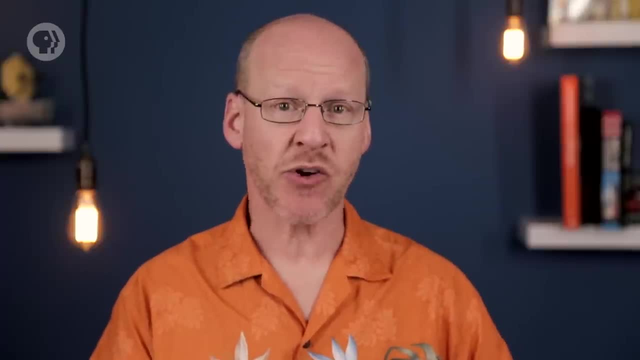 The Dutch-Italian satellite Beppo-Sax had launched the year before, designed in part to look for transient flashes of high-energy light and nail down their positions. In 1997, it detected a gamma ray burst and was able to get a reasonably decent location. 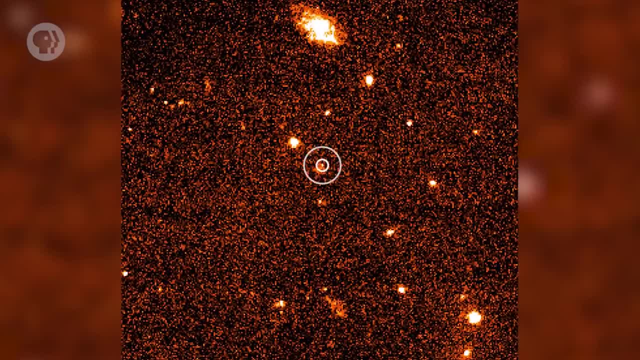 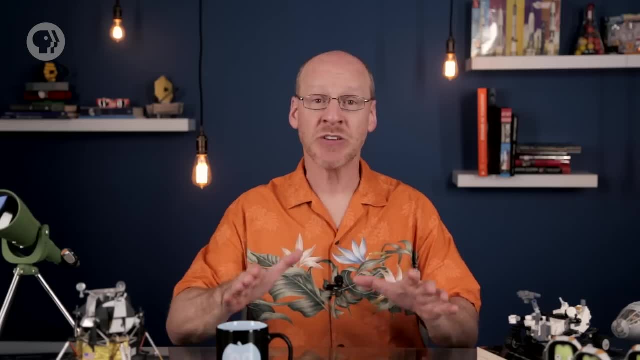 for it in the sky. Within hours, ground-based telescopes pinpointed the position and, for the first time, saw the fading afterglow of a GRB. Astronomers were stunned. The burst was clearly and obviously sitting right on top of a faint galaxy. 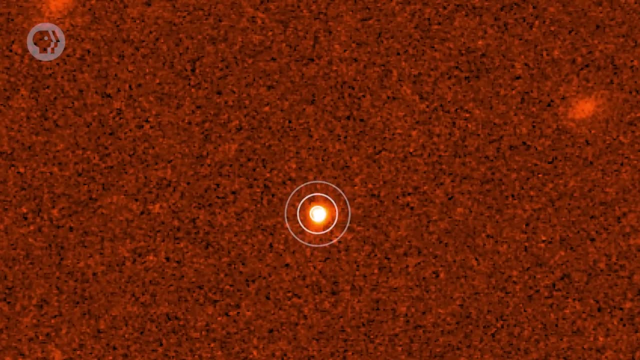 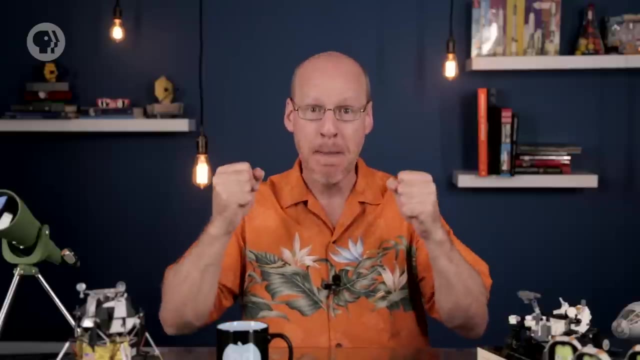 Another different GRB was detected just months later, also in a faint galaxy. When the distance to that galaxy was found, astronomers were shocked again. It was a truly staggering 6 billion light years away. The mystery was over, but it was replaced by a bigger one. 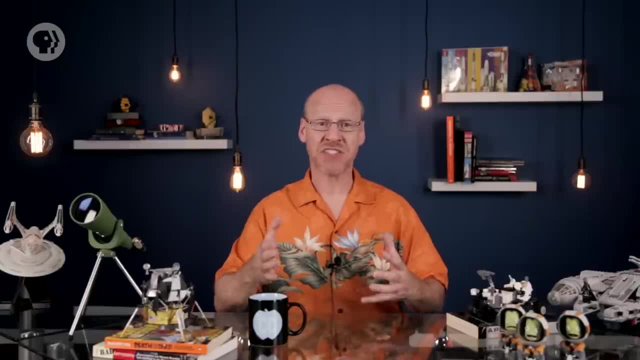 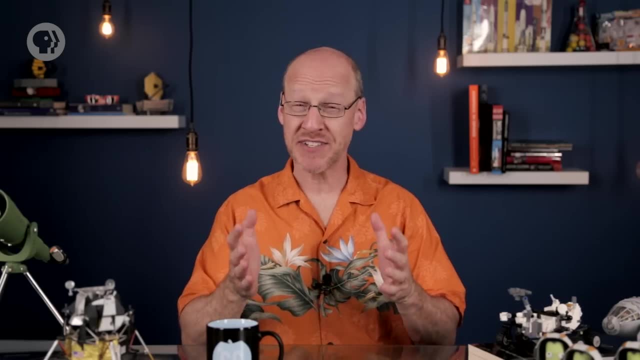 These things were happening incredibly far away, But that meant they must be unbelievably powerful. What could cause such a catastrophe, A catastrophic explosion? When you need raw power, a good place to look is a black hole. Those are created when the cores of massive stars collapse and the stars explode. 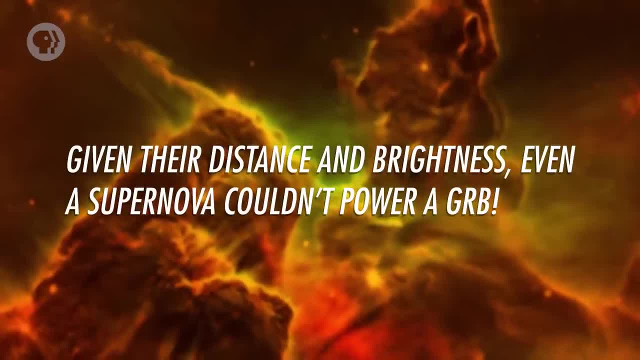 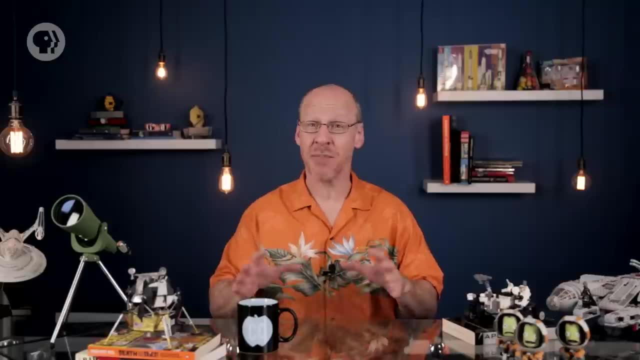 But there's still a problem. Given their distance and brightness, even a supernova couldn't power a GRB. Think about that for a second. The most violent known events in the universe at the time were inadequate to explain the ferocity of a gamma ray burst. 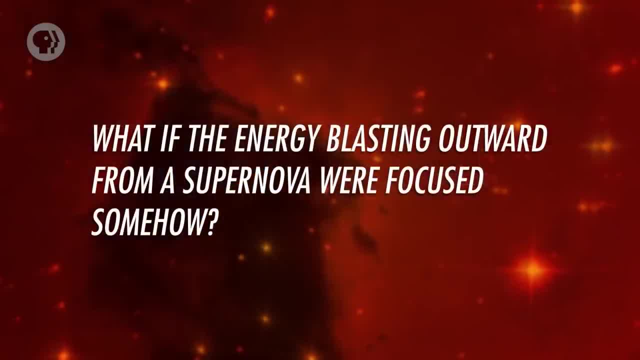 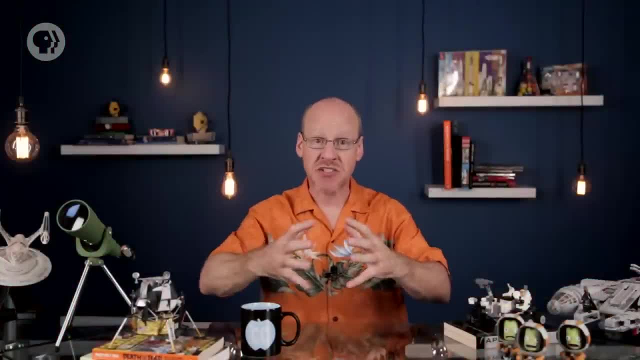 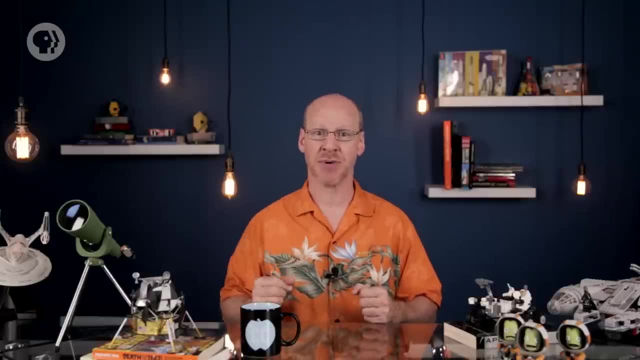 Unless…. Astronomers came up with an idea. What if the energy blasting outward from a supernova…. …were focused somehow? In a supernova? the energy gets flung out in all directions, expanding as a sphere. If, instead, that energy could be collected and sent out as a beam, that could explain. 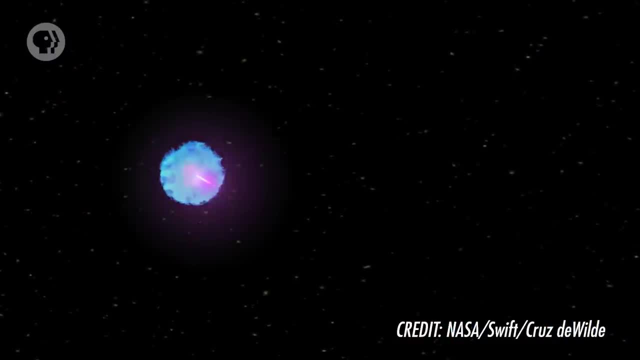 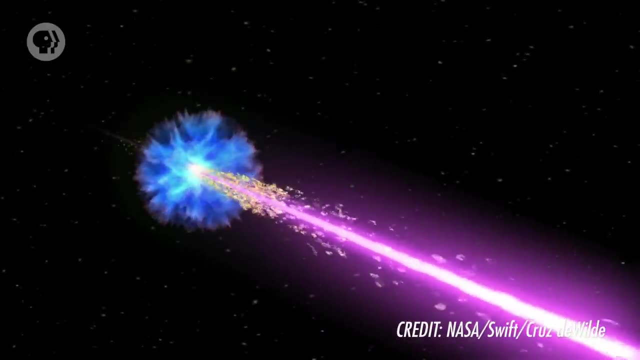 the bursts. We now understand this to indeed be the case. When the core of a very massive star collapses, forming a black hole, the material just outside the core falls down, forming an incredibly hot, swirling maelstrom called an accretion. 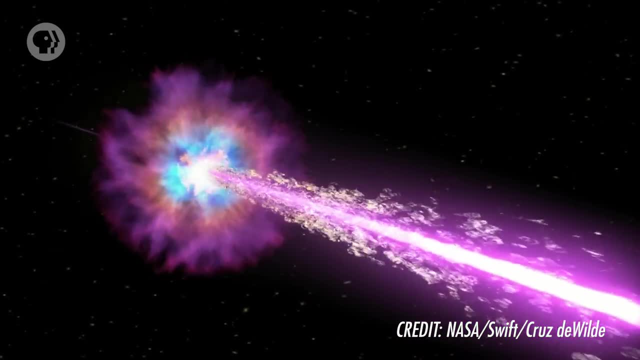 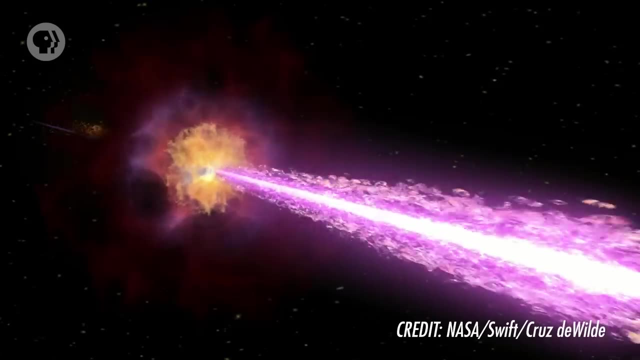 disk, The magnetic field of that material and from the black hole coil around, Wound up by the rapidly spinning disk pointing up and down out of the disk and away from the black hole. The details still aren't entirely clear, but this launches twin beams of matter, and 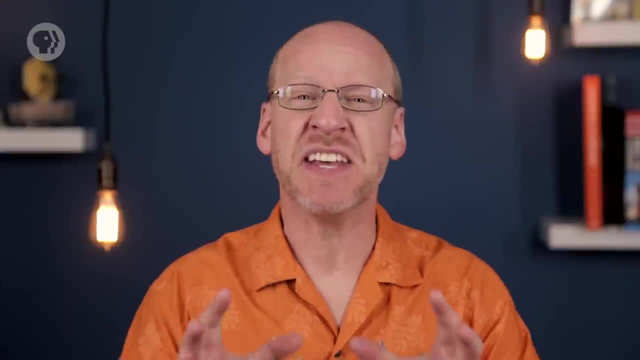 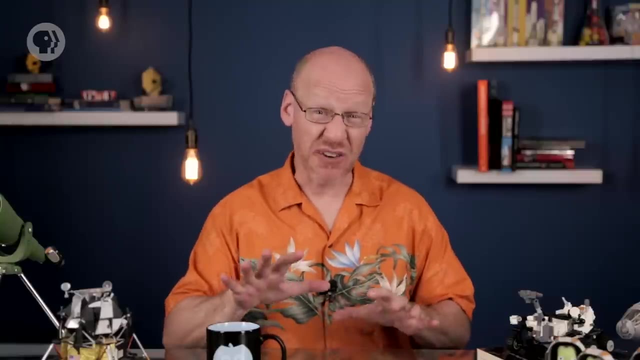 energy up and away from the black hole. The amount of energy in the beams is mind-crushing- equal to the total energy of the supernova event itself. They scream away from the black hole at very nearly the speed of light, burning through the star, blasting away across space. 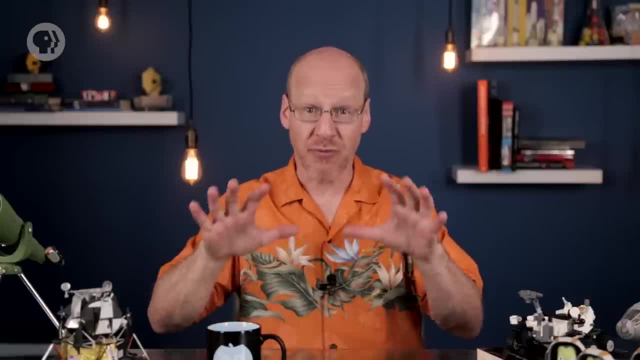 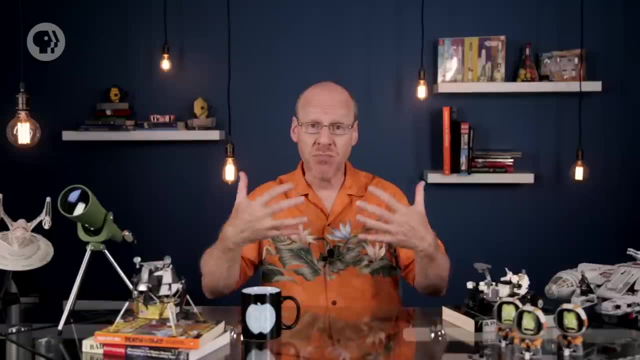 These death rays are so phenomenally bright that we can detect them from billions of light-years. We can even see the black hole from a distance. The supernova explosion is no small thing either. The star is so massive it explodes with more energy than a normal supernova. 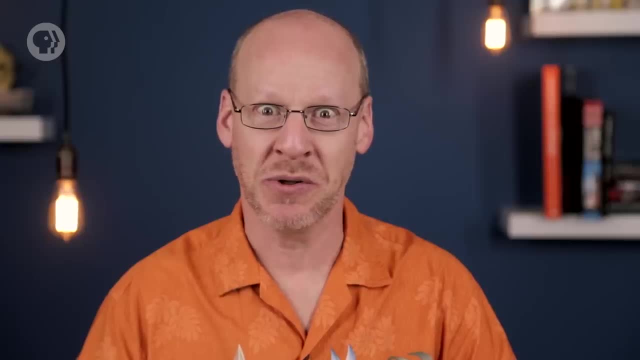 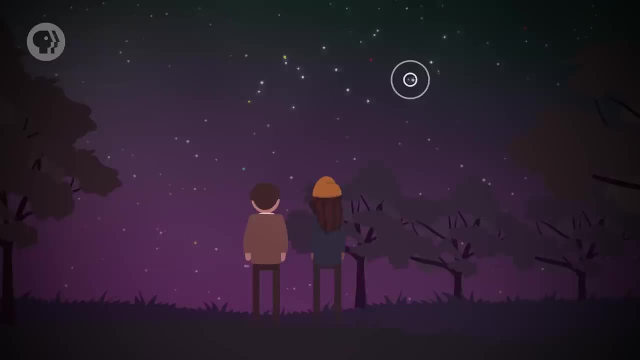 They're so powerful that astronomers call them hypernovae Cool, And you don't always need fancy equipment to see them either. On March 19, 2008,, a GRB erupted into view and its distance was quickly determined to. 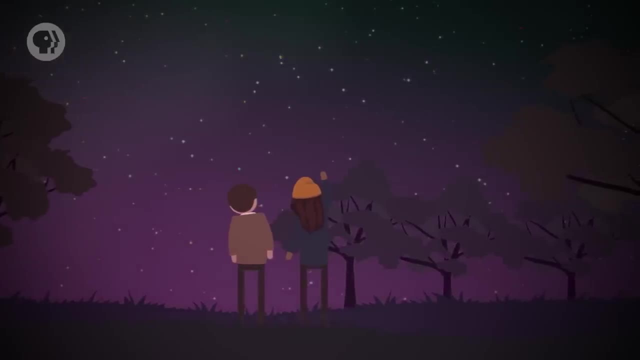 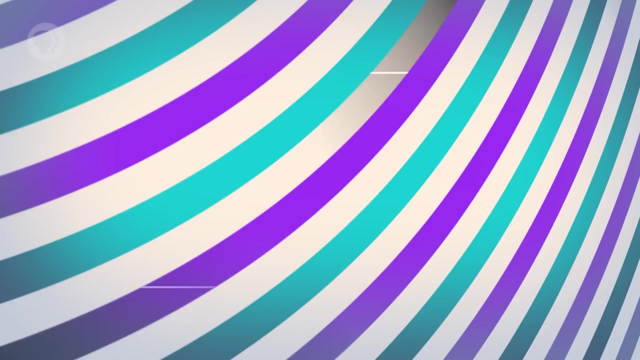 be 7.5 billion light-years from Earth. Despite that ridiculous distance, it got so bright that if you had happened to be looking at that part of the sky… You would have seen it with your naked eye. It's thought that in this case, the beam was aimed almost precisely at us, which is 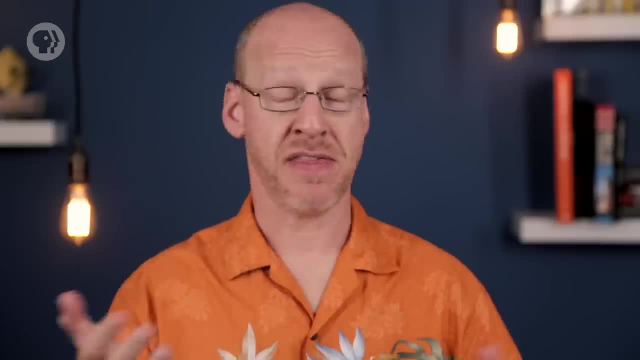 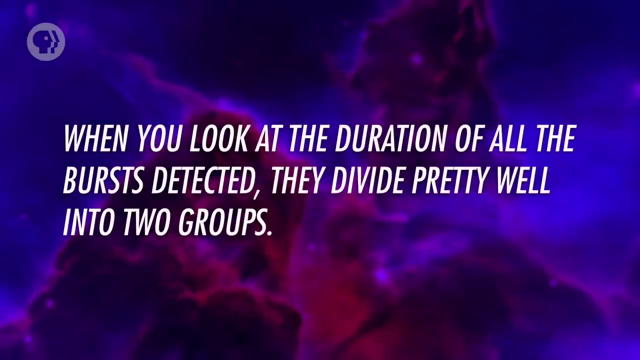 why it got so bright. Good thing it was so far away. And that explains gamma-ray bursts. Well, one kind of burst at least, It turns out. there are two kinds. When you look at the duration of all the bursts detected, they divide pretty well into two. 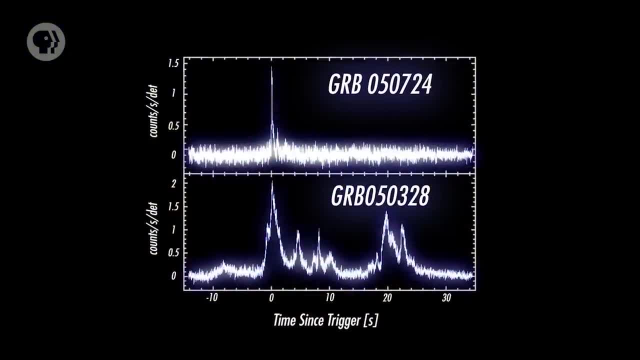 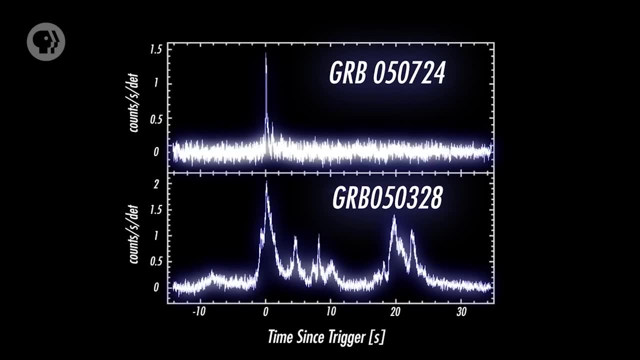 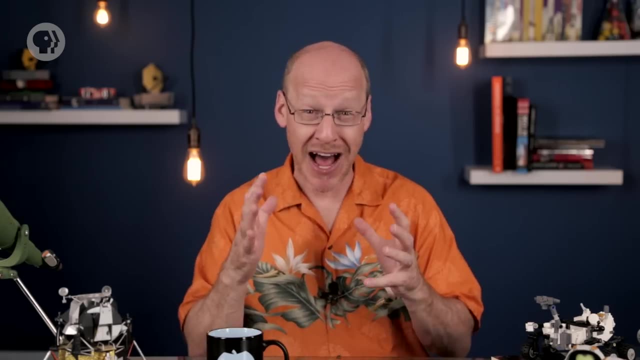 groups — ones that last longer than two seconds and come from hypernovae, and ones that are much more rapid. Sometimes these short bursts last literally four million seconds. That's why they're called hypernovae, But what else could be as soul-crushingly energetic as the explosion of a hypernova? 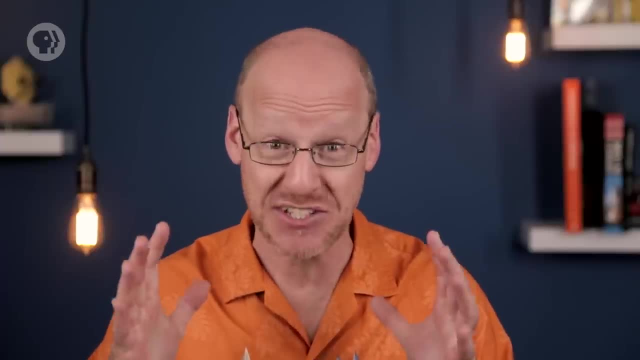 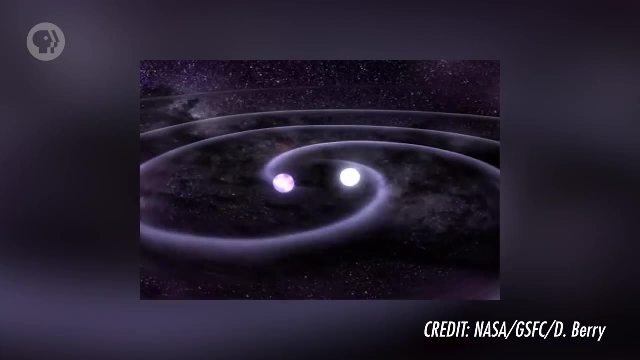 Turns out it's two neutron stars crashing together and exploding. Imagine two massive stars born together as a binary star. Eventually, one goes supernova as does the other, leaving two neutron stars orbiting each other. They'd stay in orbit like this forever if it weren't for a subtle aspect of gravity. predicted by Einstein's theory of relativity. Massive objects revolving around each other very slowly lose orbital energy by radiating away gravitational waves — essentially ripples in the fabric of space itself. I know it's weird, Relativity is like that. But think of it as a slow leak in the orbits, very gradually dropping the neutron stars. 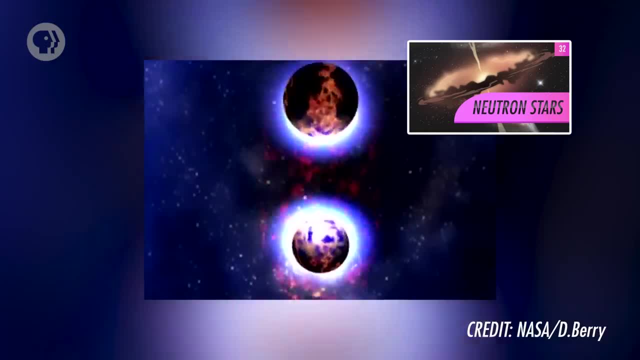 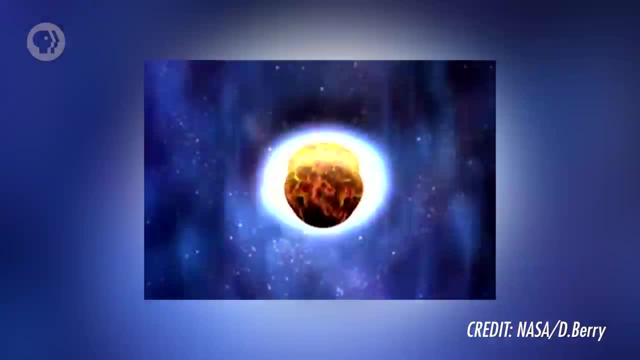 together Over billions of years. the two stars draw ever closer. getting so close they spin madly around each other. Finally, they merge in a flash, Literally. If their combined mass is more than 2.8 times that of the Sun, they'll collapse to form. 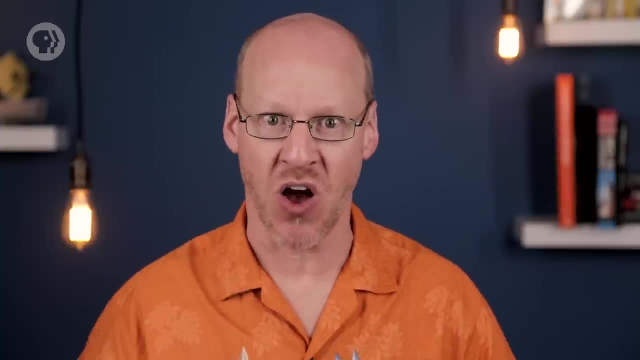 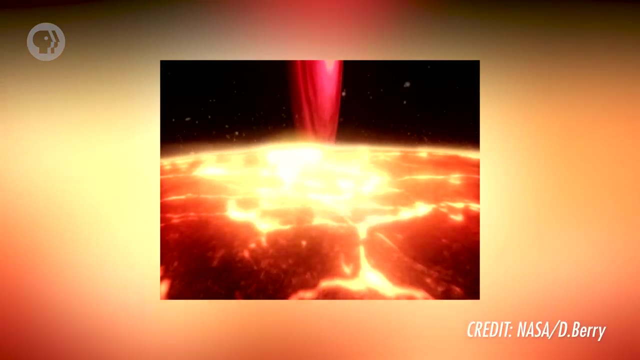 a black hole. What happens next is as bizarre as it is awesome. For a very brief moment, the system becomes a black hole orbited by ultra-dense debris from the merger- A huge amount of neutronium, neutron, star stuff. This then mimics what happens in a hypernova. 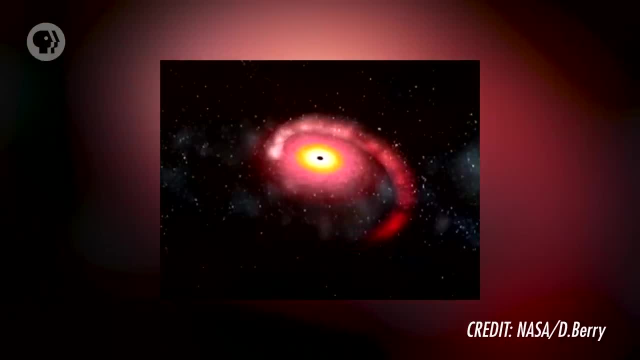 It becomes an accretion disk, heated to ridiculous temperatures, blasting out those beams of matter and energy. Because the material is more compact, the gamma-ray flash is much shorter. In case you're wondering, the gamma-ray flash is much shorter. 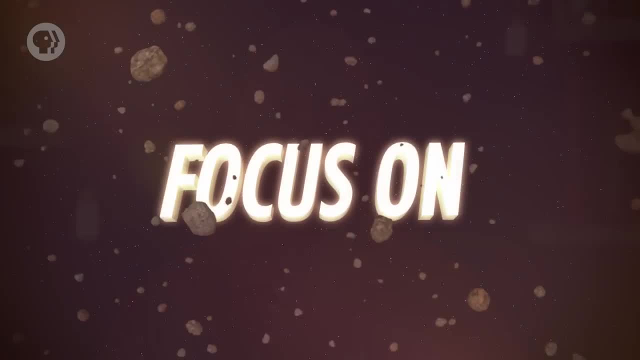 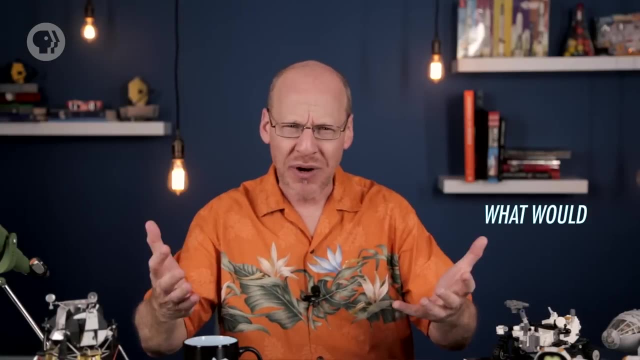 In case you're wondering: yes, this is precisely what my nightmares are made of, Which brings me to this week's Focus On If GRBs are so explosive- we can see them from halfway across the universe. what would happen if one were nearby? Well, not good things. I already talked about the dangers from a nearby supernova, and the dangers from GRBs are about the same. However, because the energy is beamed, GRBs are dangerous from much farther away. A supernova has to be only a few hundred light years away to hurt us. But a GRB can be over 7,000 light years away and do the same amount of damage. But there's an upside to those beams. Because they're so narrow we can only see a burst if the beam is aimed right at us. 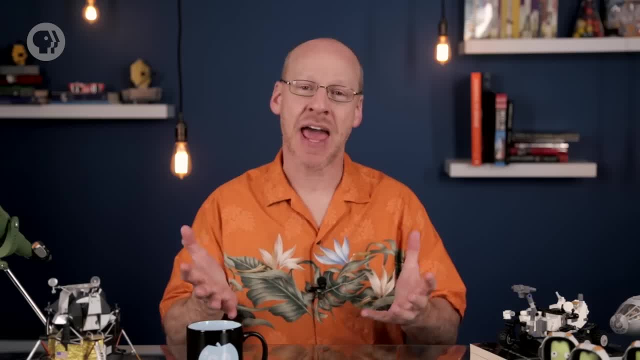 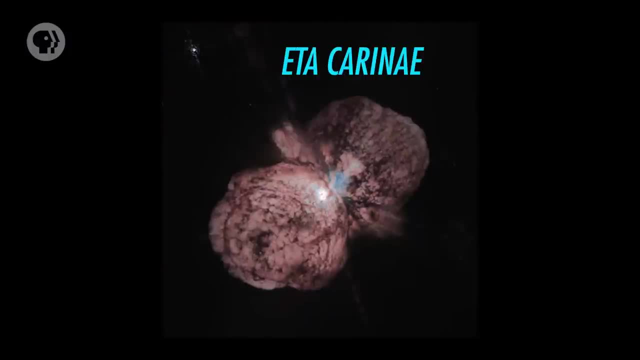 That significantly lowers the chances of getting hit by a nearby one. As it happens, there are two stars that could one day explode as gamma-ray bursts that are within the danger zone: Eta Carinae and WR104.. The good news is that both are at the edge of that distance limit, so they probably can't hurt us. 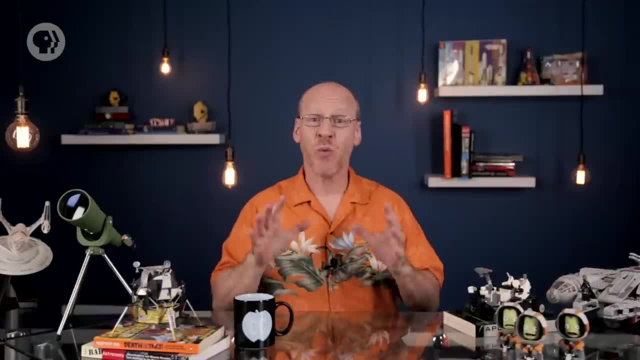 Even better, it doesn't look like either of them is aimed at us. As far as we know, we're safe from hypernova-induced GRBs. We don't know of any about-to-merge neutron stars either. It's possible they'd be dark and difficult to detect, but they're so rare that it's. incredibly unlikely that any are nearby. Because of this, I'm not really worried about them. Over the years, more space observatories have been launched to detect bursts. Probably the most important observatory is NASA's SWIFT, designed to detect the flash. 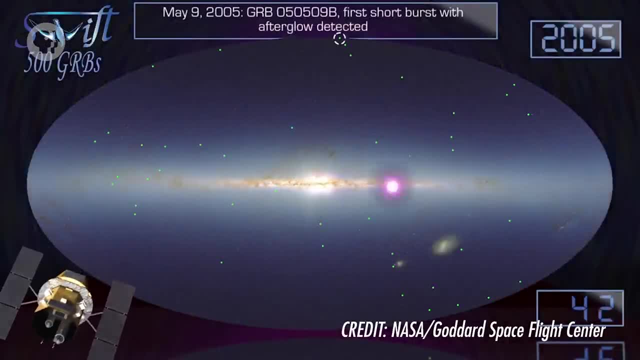 of gamma rays from a burst then swing rapidly into atmosphere. It's the largest observatory in the world. It's the largest observatory in the world. It's the fastest in action to point its ultraviolet and optical telescopes at the area precisely. 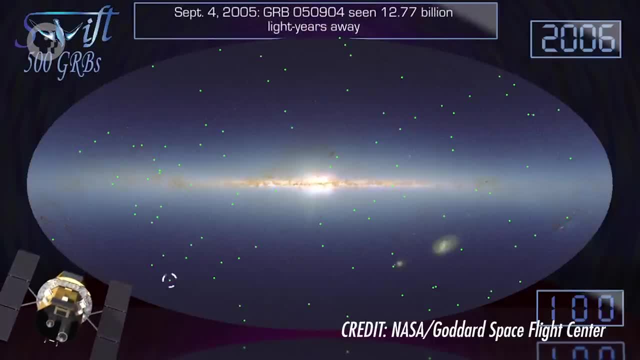 locating the burst. It then sends the coordinates down to Earth so that more telescopes on the ground can join in on the fun. As of 2015,, SWIFT has detected over 900 GRBs. The rapid response time is critically important in getting follow-up data of the bursts. 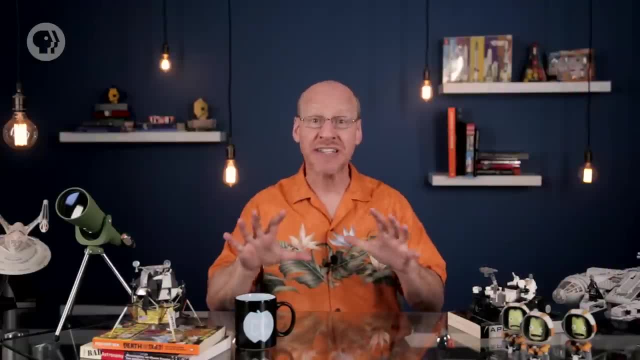 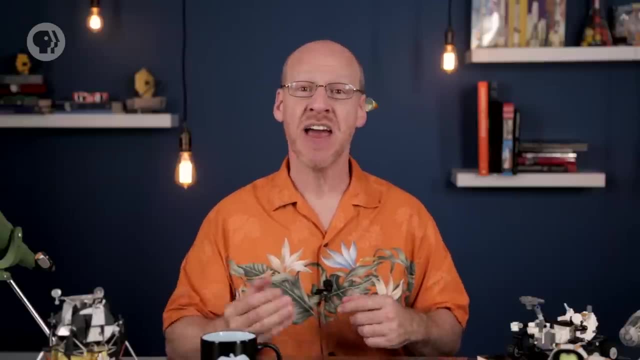 And since the launch of SWIFT, our understanding of these phenomena has grown by leaps and bounds. Now, with our fleet of satellites scanning the skies, we see a GRB pretty much every day. And remember, We only see them when they're aimed at us. 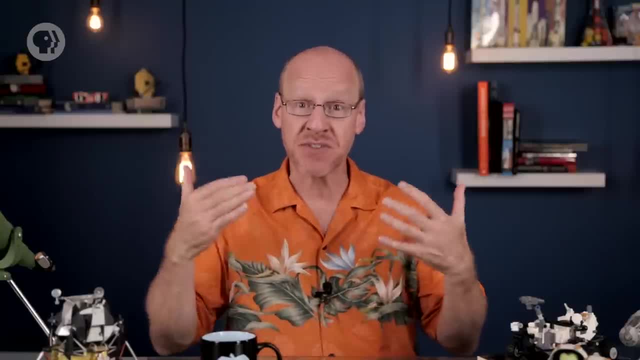 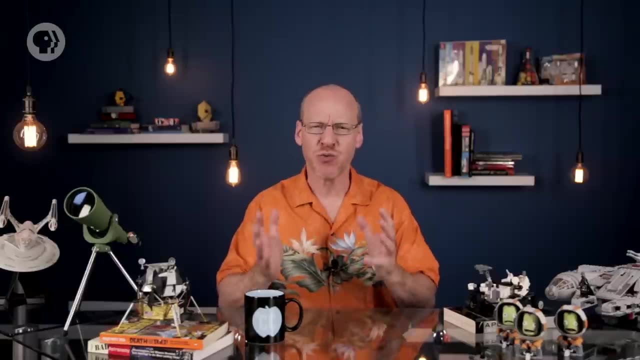 That means we miss most of them, so the actual rate of GRBs is much higher. in the Universe There may be hundreds happening every day somewhere in the cosmos. Gamma ray bursts are truly one of nature's most incredible events, the most violent and 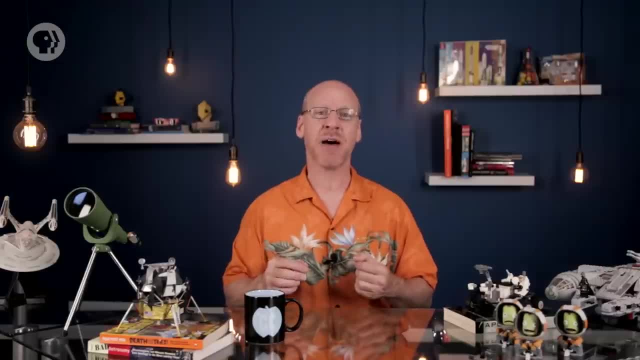 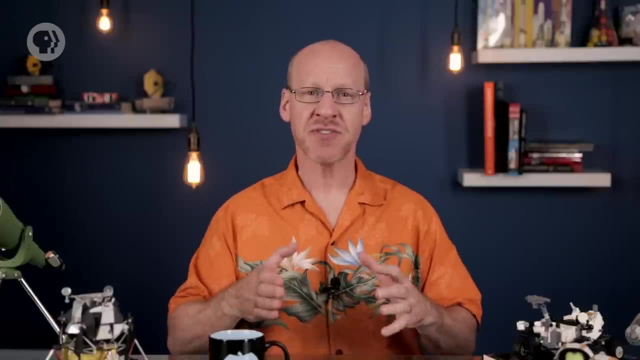 energetic explosions the Universe is capable of. Everything about them is amazing, from their discovery to what actually powers them and what they create. In fact, when you think about it, here's the most astonishing thing about them. Every time we see one, we're witnessing a black hole being born. 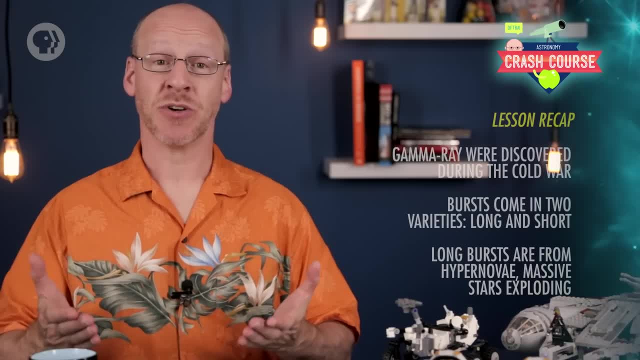 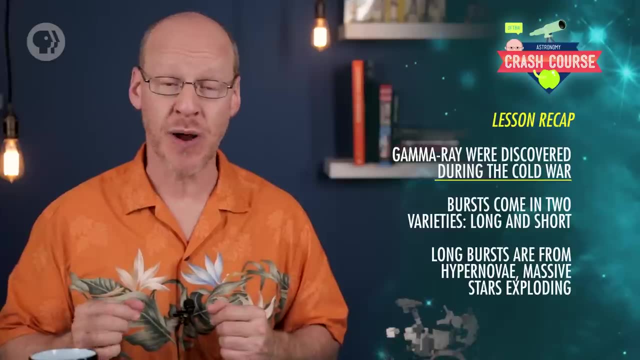 Gamma ray bursts are the birth cries of black holes. Today you learned that gamma ray bursts were discovered during the Cold War, when both the US and USSR were worried about the other group detonating nuclear weapons in space. Bursts come in two rough varieties: long and short.